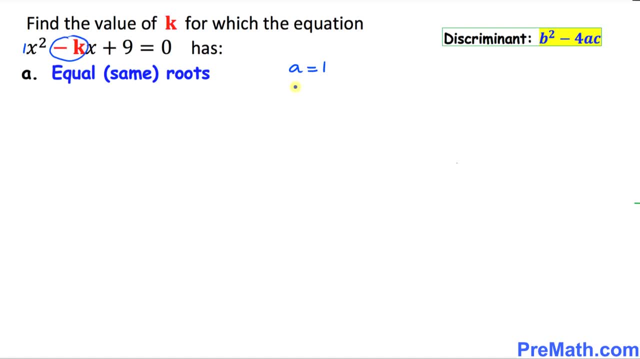 to one. and here our b, a negative K and C is simply 9. so it has two equal or same roots if the discriminant equal to 0. so let's fill in the blanks. I'm going to put down: B square minus 4, AC equal to 0. we know our a equals to 1, B is negative 4. I'm going. 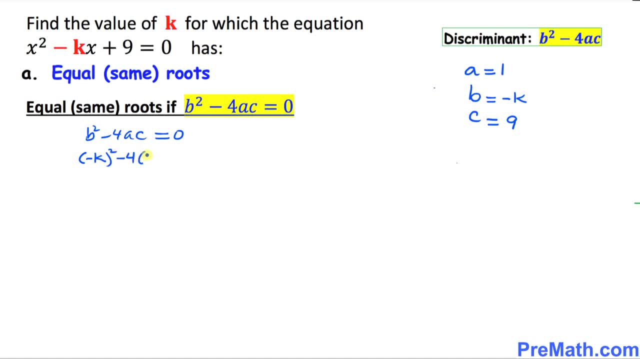 to say negative 4 square minus 4, time a is 1 and C is 9, equal to 0. let's simplify this: simply become K square minus 36 equal to 0. let's move this 36 on the other side. let's move this 36 on the other side. 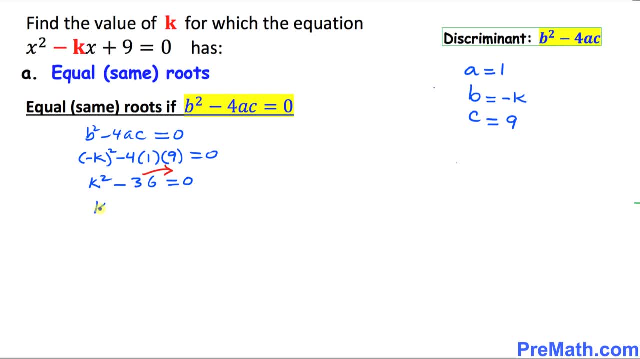 so this simply is going to become K square equals to 36. let's take care of this one over here. undo this square by taking the square root, so that is going to give us simply K equal to positive or negative 6, so thus K equal to negative 6. 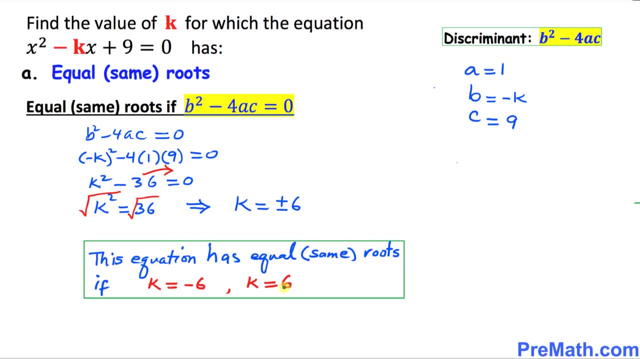 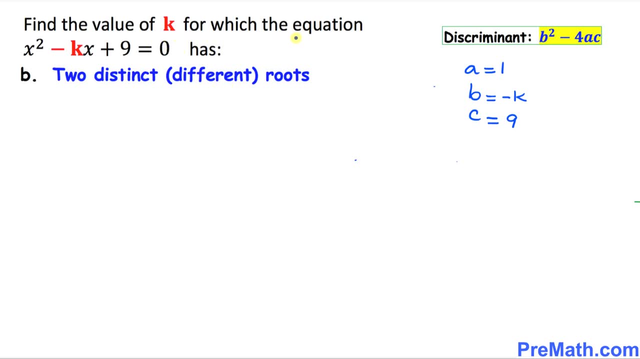 and K equal to 6 is our answer. and here is in the next part, we have to find the value of K for this given quadratic equation if it has two distinct or different roots. so this condition happens only if this discriminant B square minus 4 AC is. 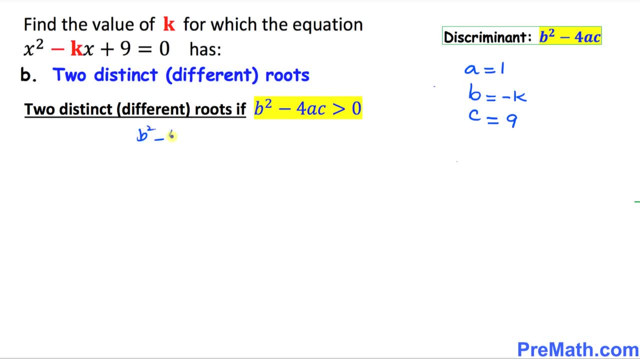 greater than 0. let's fill in the blanks. b square minus 4 ac is greater than 0. in our case, b is simply negative. k square minus 4 times a is 1, c is 9 is greater than 0, so they simply become: k square minus 36 is greater than 0. 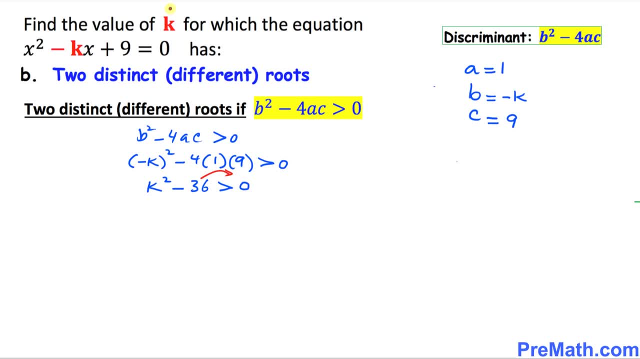 let's move this 36 on the other side. so we simply got k square is greater than 36, and if you have this kind of scenario, when you have inequality greater, then this tells you that k is is less than negative 6 or k is greater than 6. so now you might be wondering: why did I put this way? k is. 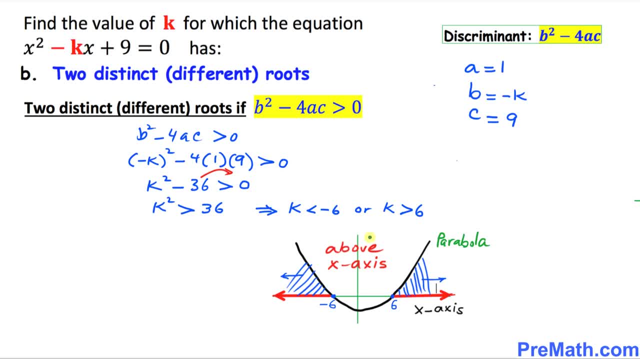 less than negative, 6 or k is greater than 6. let me just give you really quick kind of explanation over here, as you can see that this k square minus 36, this represents this kind of graph. this is called parabola. okay, so this is a. 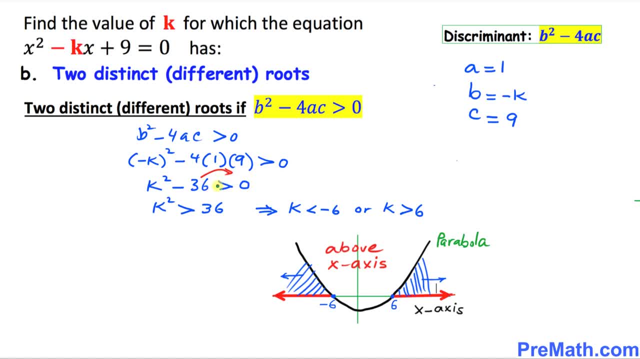 parabola and since this parabola, this is greater than 0. you can see over here. greater than 0 means that means we are above xs. look at the above x is shaded region. that means these two arrows are going in the opposite direction. one is going on the left hand side of this negative 6 and the other 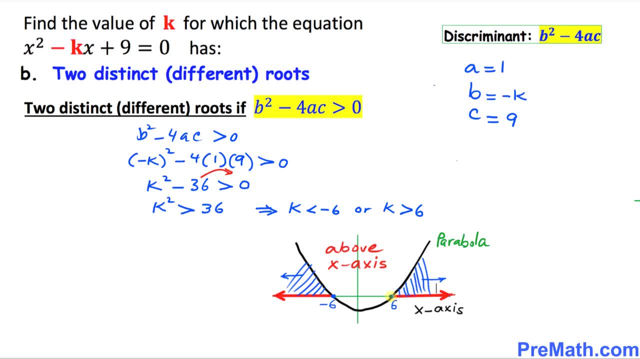 one is going right hand side of this positive 6. no wonder I put down k is less than negative 6 for left hand side. and for right hand side I put it down k is greater than 6 and I put an or because they are in opposite. 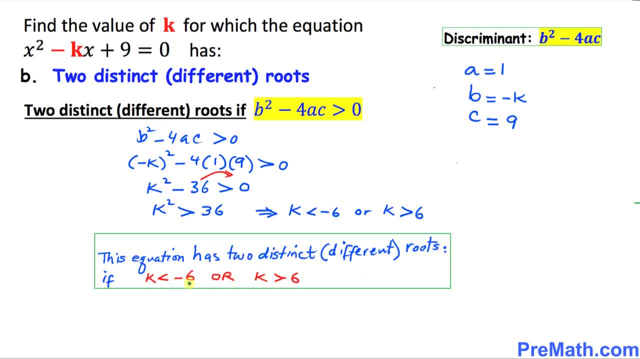 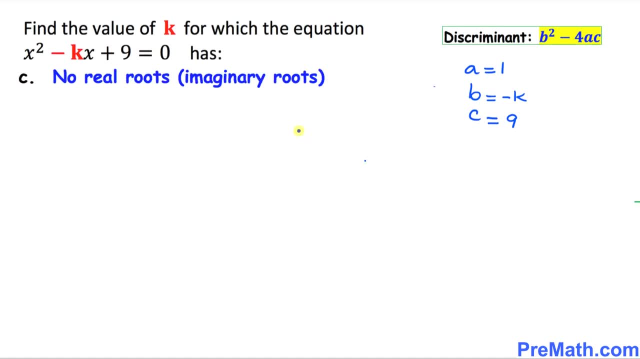 they are disjoint and thus k is less than negative. 6 or k is greater than 6 is our answer, and in this part we have to find the value of k, and the condition is that this quadratic equation has no real roots. no real roots means that 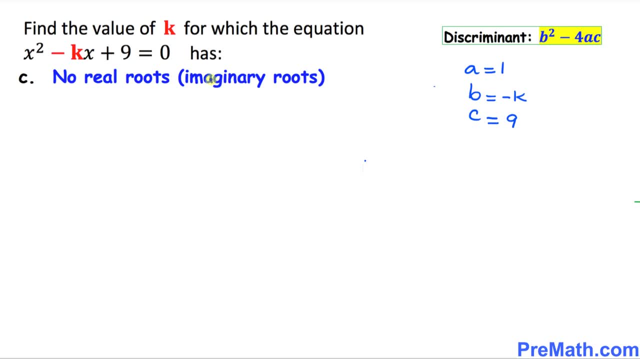 then it's going to be imaginary roots. then, and in this case the discriminant must be less than zero to get a, no roots. so let's simplify this one. I'm going to put down b square minus 4: ac is less than we know, b is negative k. then put down, square minus 4 times, a is 1, c is 9, less than zero. let's. 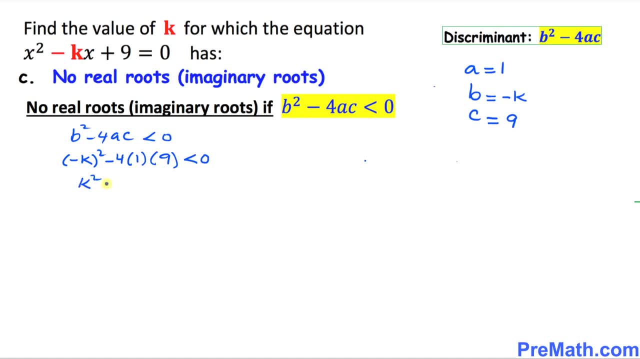 simplify this. simply become: k square minus 36 is less than zero. make sure we are dealing with inequality. I want you to move this 36 on the other side, so this is going to give you k square is less than positive 36.. If this is the scenario, then we know that this is going to be. 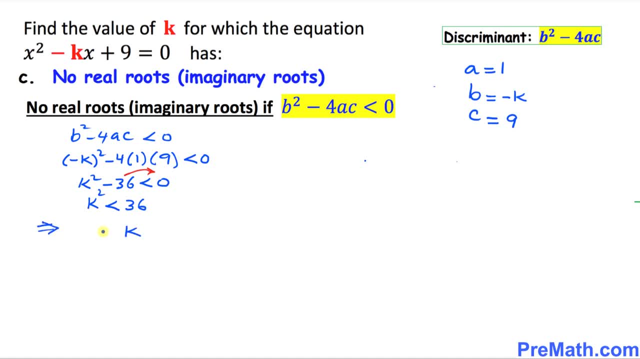 simply k is going to be in between negative 6 and positive 6.. And you might be wondering: how did I get these inequalities? Let me just show you once again that this graph, this function, represents this graph called parabola. Since now you know that this is less than 0 means that means. 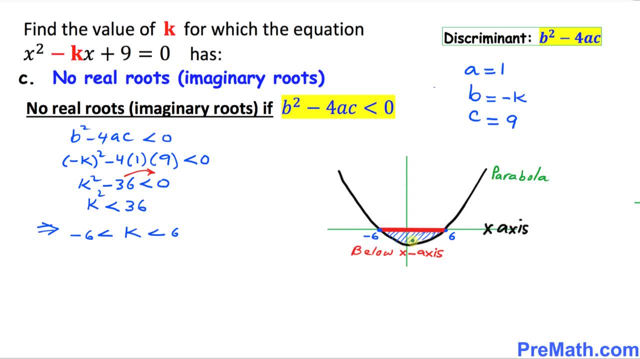 the graph. we are looking at it below x axis, So the below axis shaded region is only this part. So this is restricted between negative 6 and positive 6.. So 0, 0, 0, 0 0- no wonder I just put a k- is restricted between negative 6 and positive 6.. This is just like a. 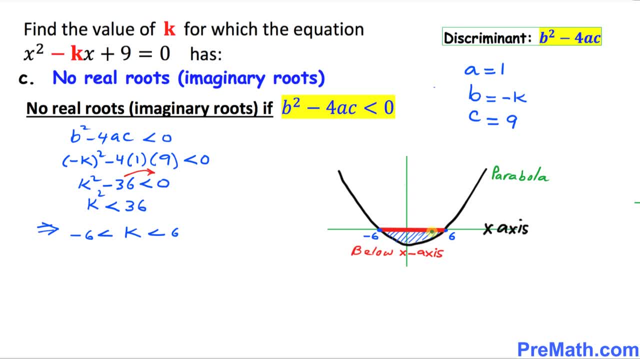 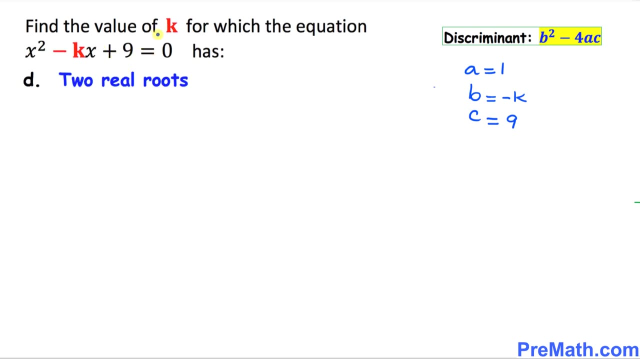 sandwich between negative 6 and positive 6.. So thus our answer turns out to be: k is between negative 6 and positive 6, and that is our answer. And finally, in this part we are going to find the value of k if this quadratic equation has two real roots. So now we have no any kind of clue. 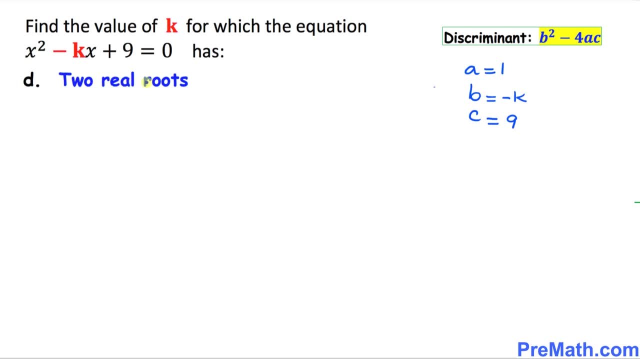 whether this is distinct or equal roots. just simply it's a little bit ambiguous. So in this case, only two real roots, then we have to apply this condition: In this case, the discriminant b square minus 4ac must be greater than 1.. 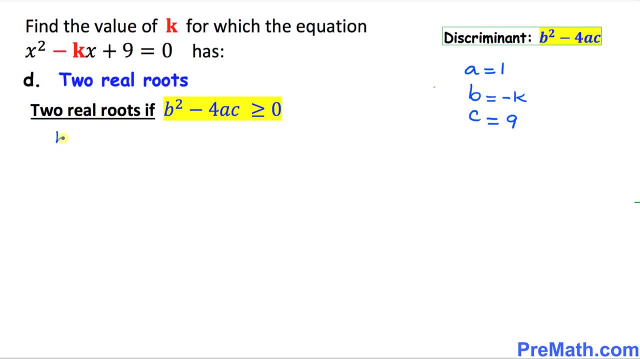 are equal to 0.. So let's get started then. I'm going to put down: b square minus 4ac is greater than equal to 0.. Let's fill in the blanks. b square means negative. k square minus 4 times a is 1, c is: